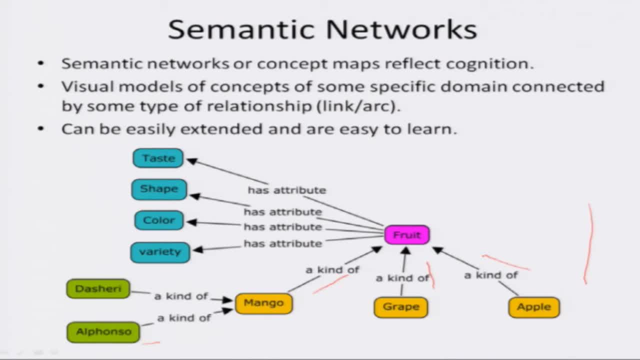 of fruit. Apple is a kind of fruit. fruit has attribute taste, fruit has attribute shape, fruit has attribute color and fruit has attribute variety. Now it is easy to see that concert maps can be visualized as a collection of object, attribute value triplets. 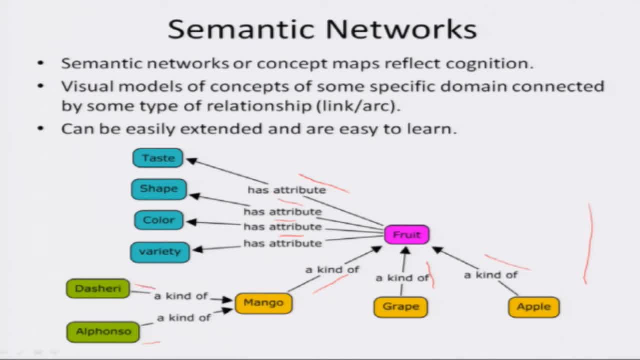 For example, the sherry has attribute a kind of that has value. mango alphonse has attribute a kind of that has value. mango mango has attribute a kind of that has value. fruit grape has attribute a kind of that has value. fruit apple has attribute a kind of that. 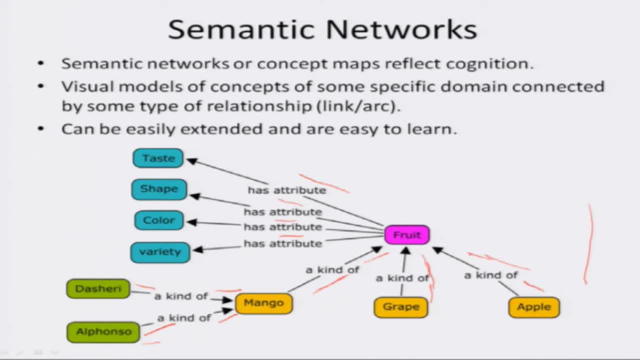 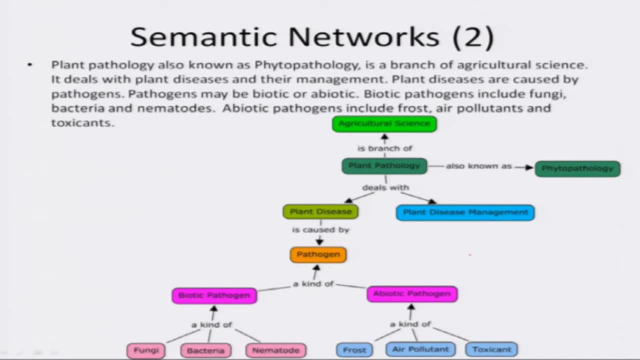 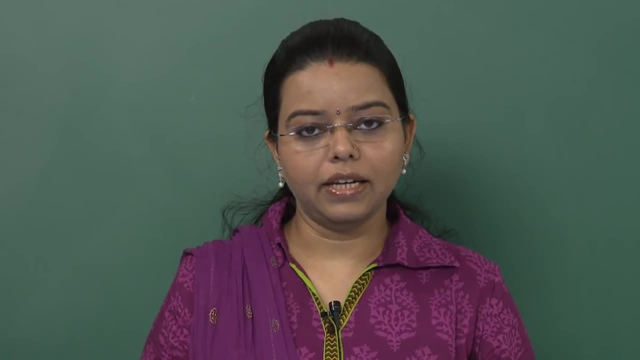 has value fruit, and same goes with other relationships as well. Now let us see how to draw a concert map map knowledge that is represented in natural language. It is a three-step process. First of all, we need to identify the concepts, and then we identify the relationships between: 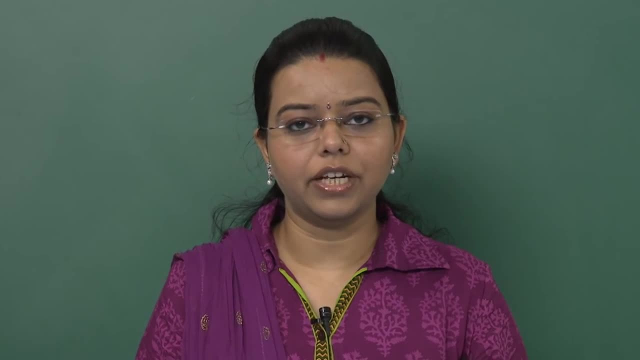 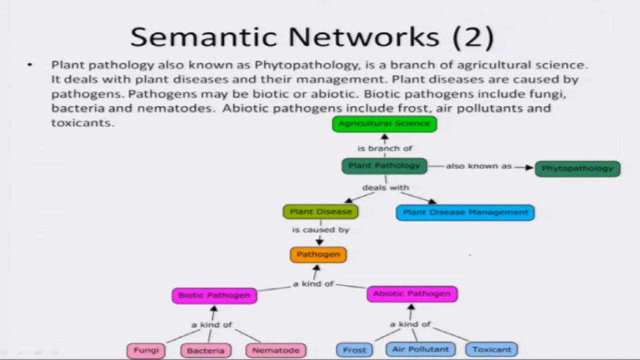 the concepts and then, finally, we plot the concepts and relationships into the concept map. For example, plant pathology is also known as phytopathology is a branch of agricultural science. Now, here the concepts are: plant pathology, phytopathology and agricultural science. We 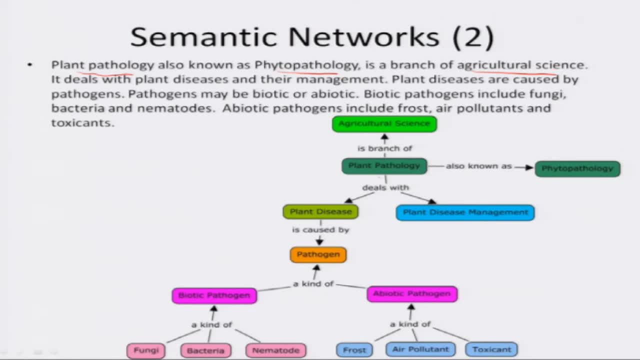 draw these concepts in the form of rectangles in concept map and finally join them with the help of the relationships between them. Plant pathology is connected to phytopathology by the also known as relationship. Similarly, plant pathology is connected to agricultural science concept by the agricultural science concept. 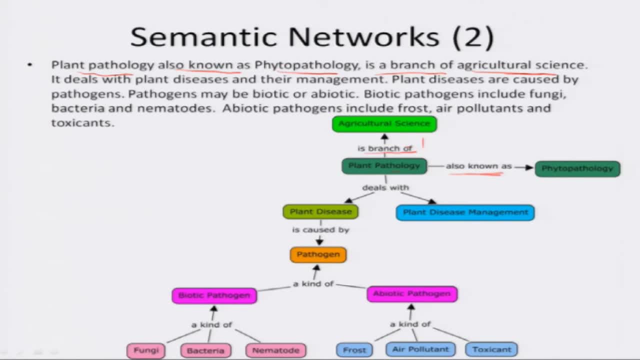 So this is branch of relationship. Then it deals with plant diseases and their management. The concepts here are plant diseases and plant disease management, So we plot them as concepts in the concept map and link them with the plant pathology concept by means of deals with relationships. Plant diseases are caused by pathogens. Here 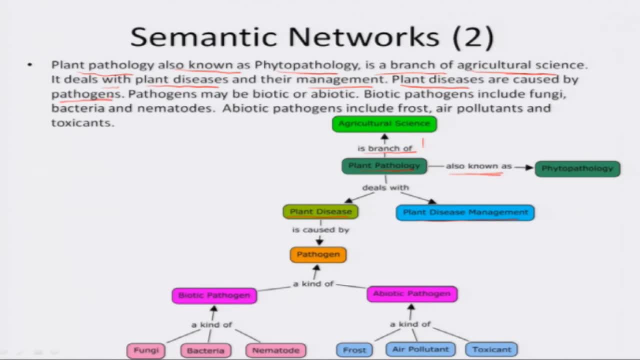 the concepts are plant diseases and pathogens. So we plot the pathogen as concept map, then we think about what pathogen is, and the principle is ANYTHING AND the issue is plant diseases, but verbatim whatいうこと. those are Enfin for записi. Switzerland analysis: this Jenna.